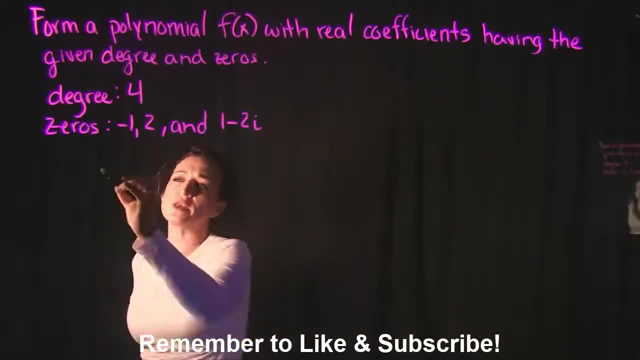 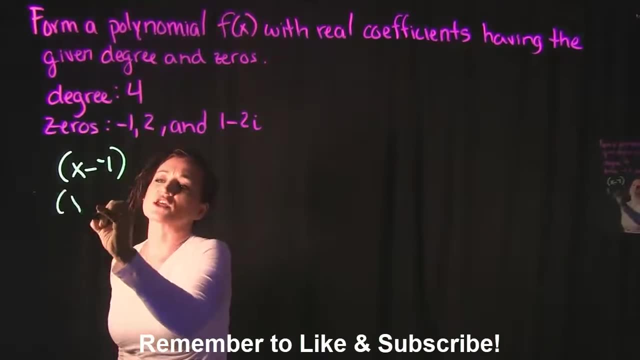 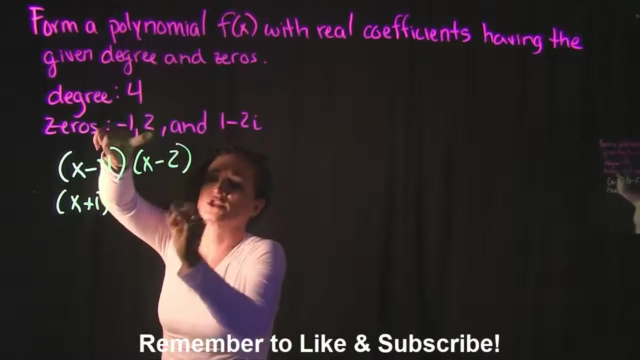 How that correlates into writing it into an equation. we need to keep in mind that we write it x minus that factor, So it's x minus the factor of negative 1, which actually turns into x plus 1.. And then we have the factor x minus 2, which is the next factor they gave us. 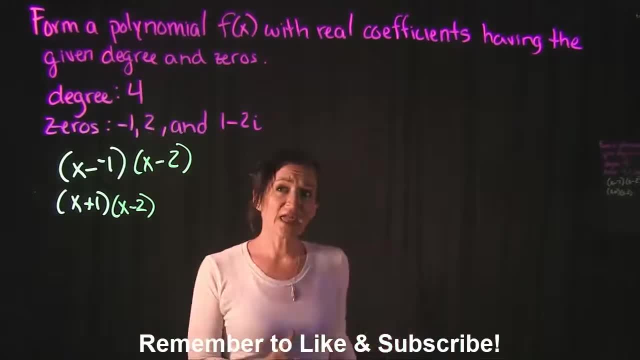 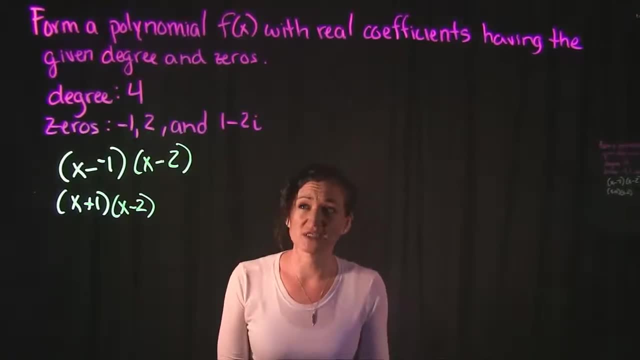 So that's just simply an x minus 2.. But then they gave us the factor 1 minus 2i. This is a complex zero here that they gave us, And when they give us a complex zero, this is what we need to do with it. 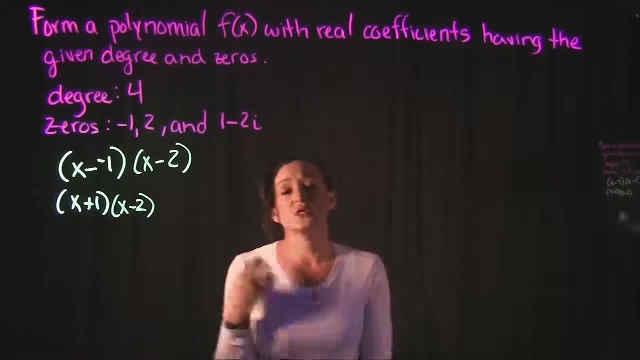 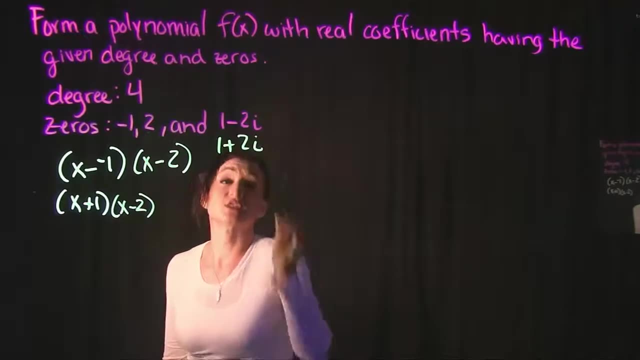 We take our 1 minus 2i, We also need to take into considering the conjugate of that. So the conjugate of 1 minus 2i is 1 plus 2i. So this is where our fourth zero comes from. 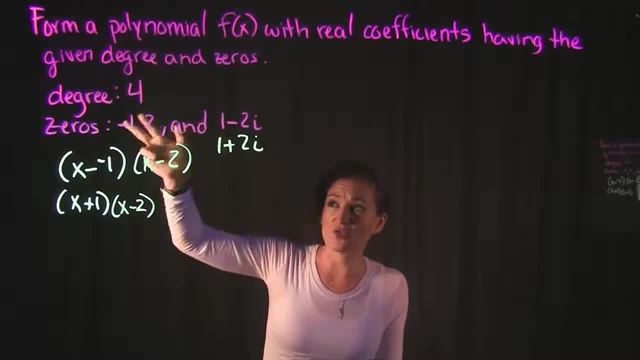 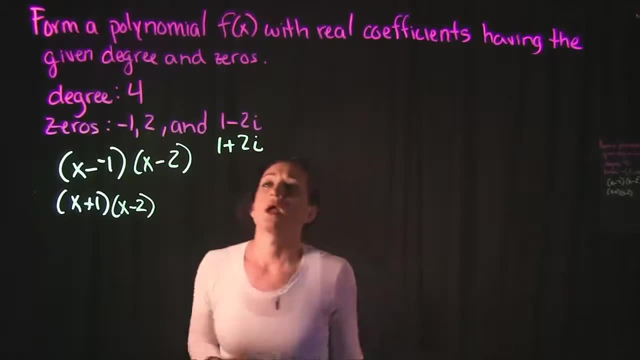 Negative. 1, 2, and 1 minus 2i are the first three And then we take the conjugate of our complex one to get our fourth zero. So we need to do actually a little bit of algebra when we do this because, remember, it's x minus that zero. 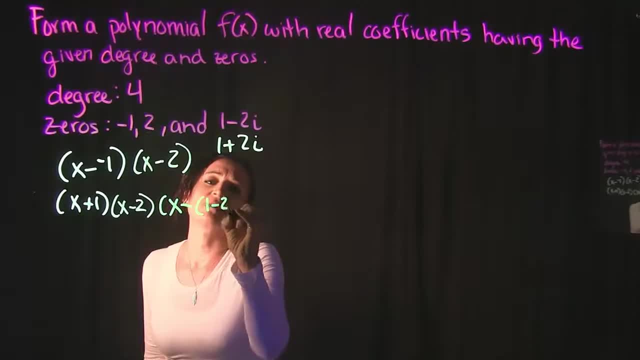 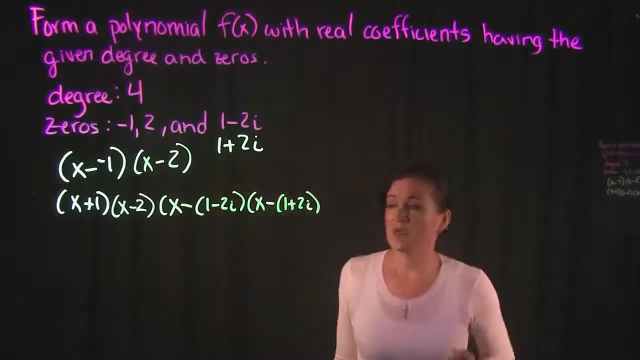 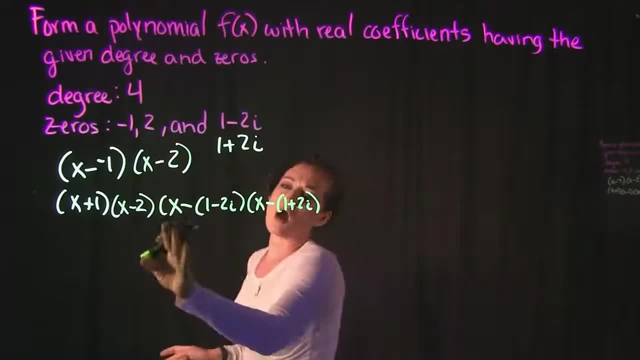 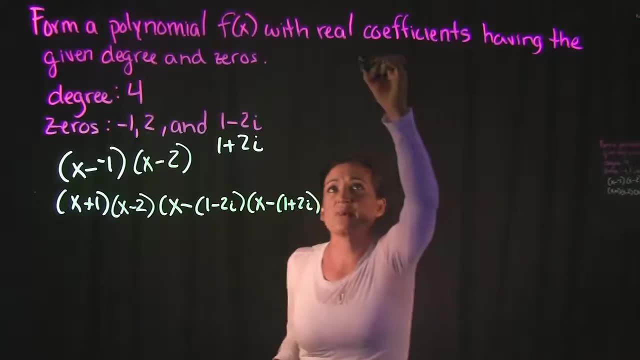 And those are going to stay, as is Our complex factors over here. we're actually going to need to do a little bit of additional work with that. We need to simplify those a little bit, So let me actually move those up here. We have x minus 1 minus 2i. 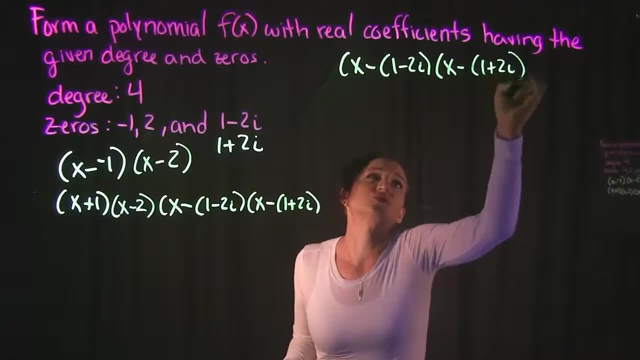 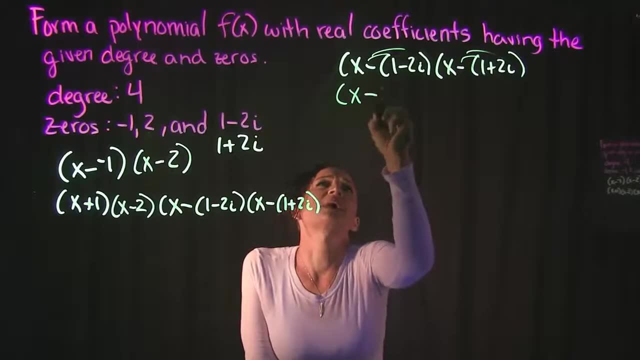 And then we have 1x minus 1 plus 2i. So the first thing I'm going to do is distribute the negative in each one of them. So if we do that, we get x x minus 1 plus 2i. 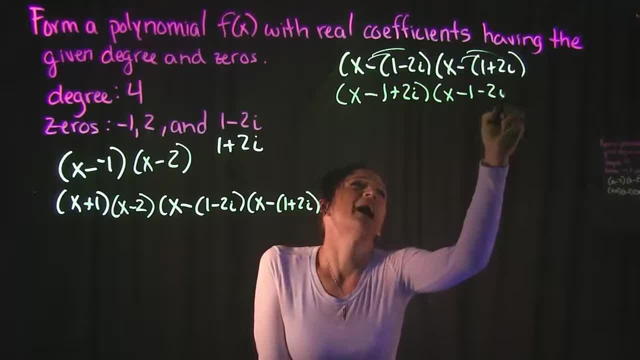 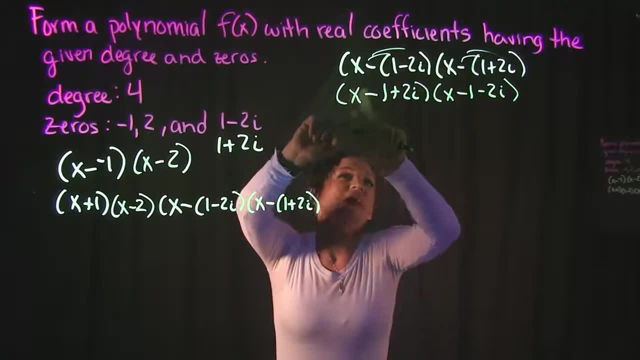 And then over here we get x minus 1 minus 2i. The next thing we need to do is we need to actually multiply this all together. So x times everything Negative, 1 times everything, 2i times everything. So let's go ahead and start that. 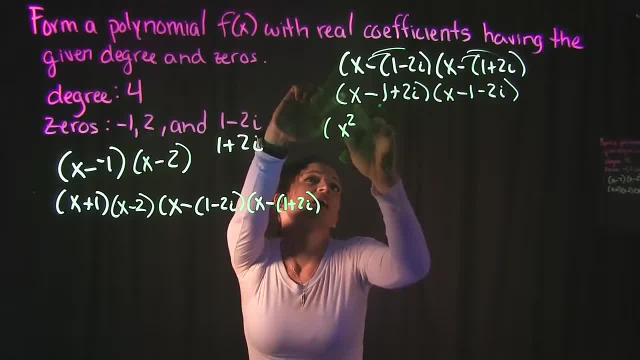 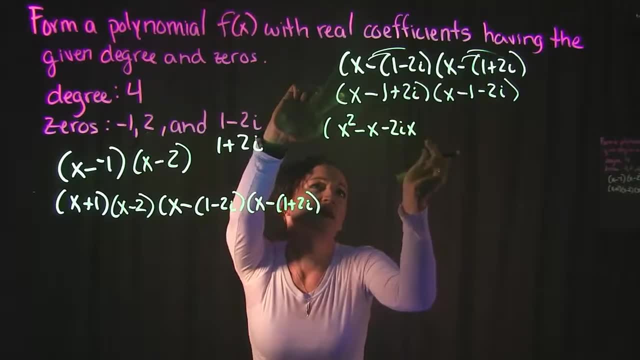 So we have x times x, which is x squared x times negative 1, which is negative x. x times negative: 2i 2i gives us a negative 2i x. Multiply everything by negative 1.. Negative 1 times x is a negative x. 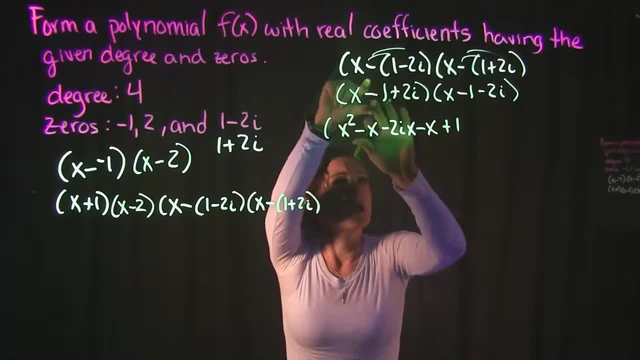 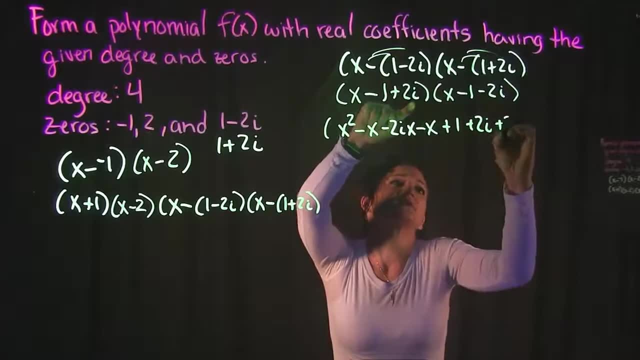 Negative 1 times negative. 1 is a positive: 1. And negative 1 times negative. 2i is a positive: 2i. 2i times everything. 2i times x is 2i, x. 2i times negative. 1 is a negative 2i. 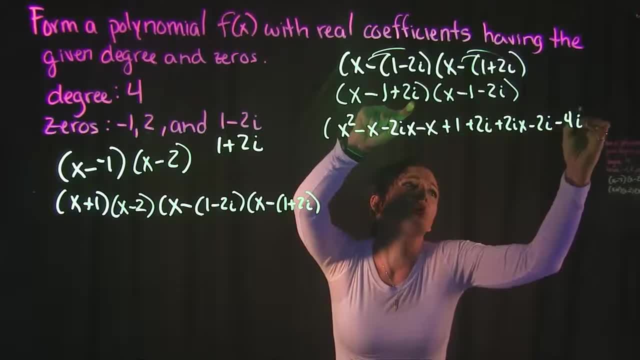 And 2i times negative 2i, that gives us a negative 4i squared, which we'll simplify here in just a little bit. Let's try and combine some light terms. So dropping down the x squared, since there's no other x squareds. 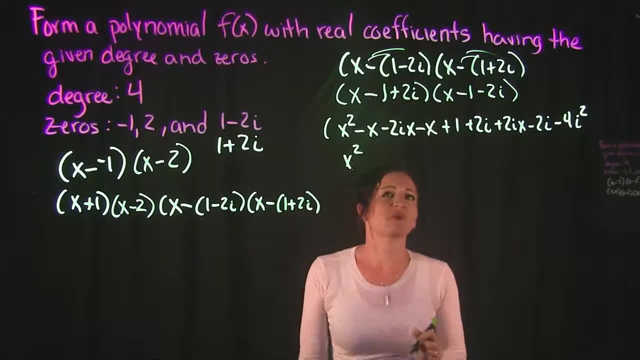 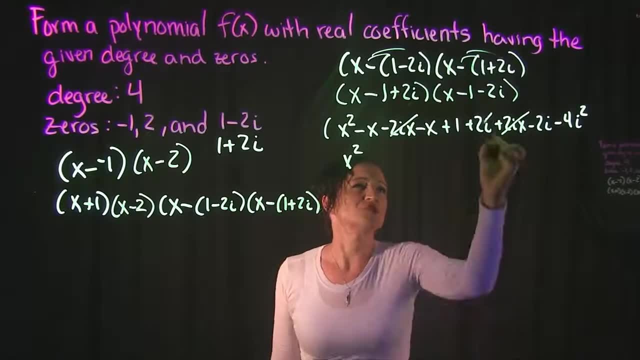 let's see what can happen here. I see that I have a negative 2i x and a positive 2i x- Those cancel. I have a 2i and a negative 2i- Those cancel. So let's see. 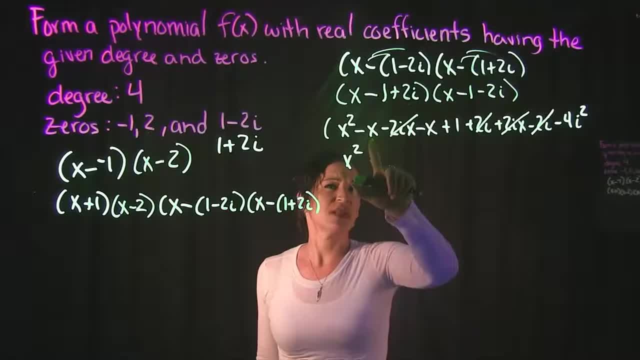 I have a negative x and a negative x, So negative x plus a negative x is a negative 2x, Right? So those are out of the way. The only thing I have left is the 1 and the negative 2i. 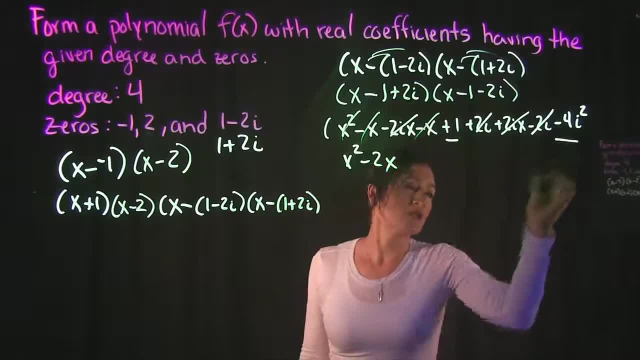 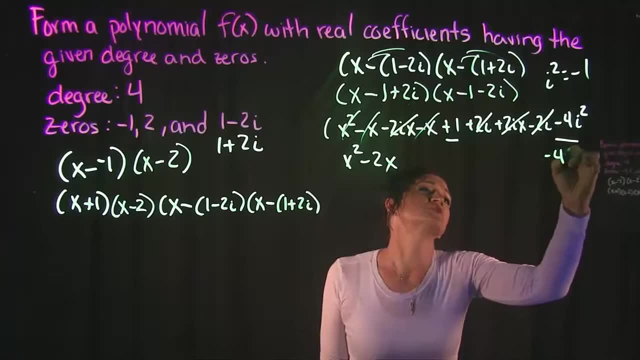 So negative x plus a negative x is a negative 2x, Right. So those are out of the way. Negative 4i squared- Remember that i squared- is equal to negative 1.. So that means that this is really negative 4 times negative 1,. 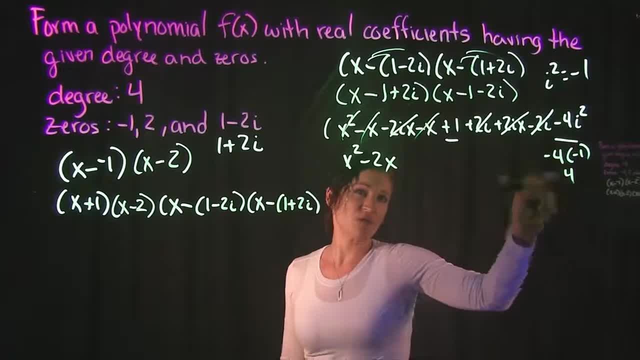 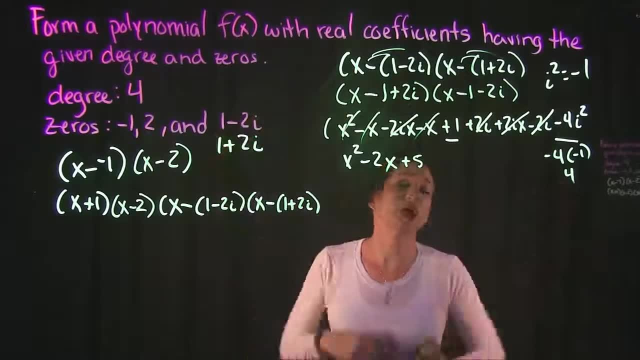 which makes this a positive 4.. So that positive 4 could get added with this positive 1 to give us plus 5.. So when we multiply and simplify these two factors together, we actually get x squared minus 2x plus 5.. 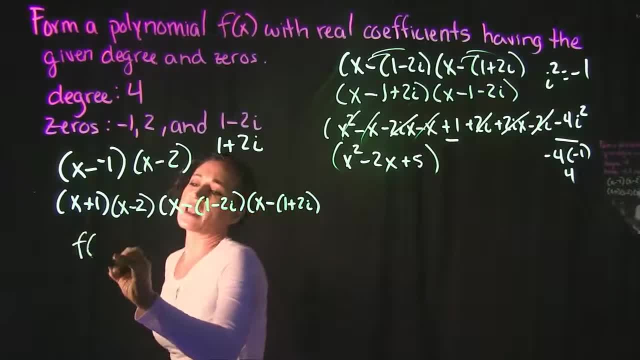 So this is what our polynomial is going to look like. It's going to look like: f of x is equal to x plus 1 times x minus 2 times x, squared minus 2x plus 5.. This should be our polynomial, right here. 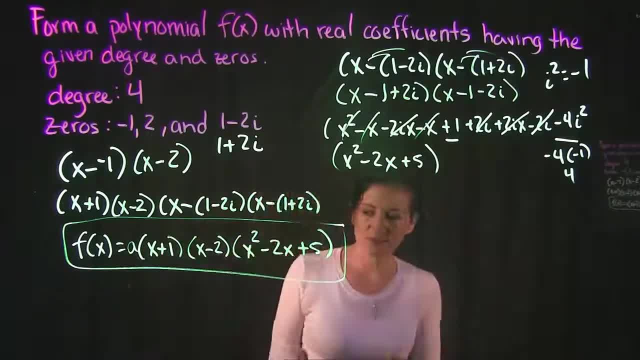 Sometimes they include the a here in the front. That's part of the formula for this particular problem. We're not solving that. It's just part of the formula, and it could be there, Though technically we could plug in a 1 for that if we wanted to.